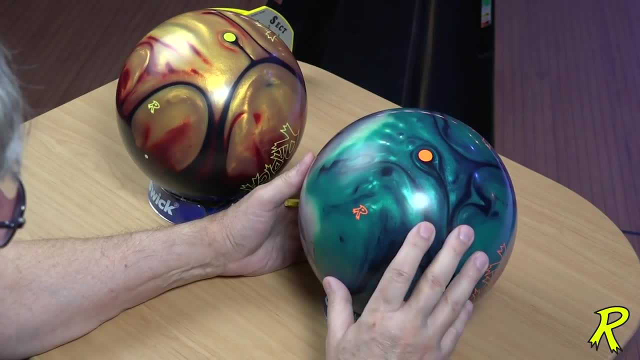 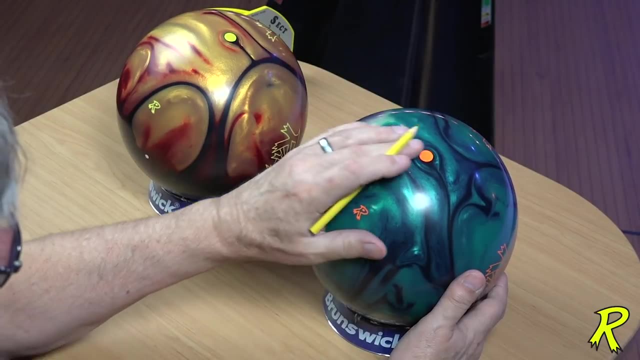 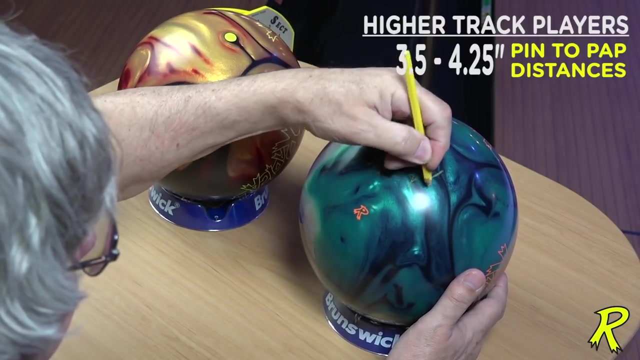 is going to be in the thumb hole When we're talking about pin to PAP distance. we're more interested in whether you are a higher track or a lower track player. Higher track players: you want pin to PAP distances between 3 1⁄2 and 4 1⁄4 inches. Okay, If you happen to. 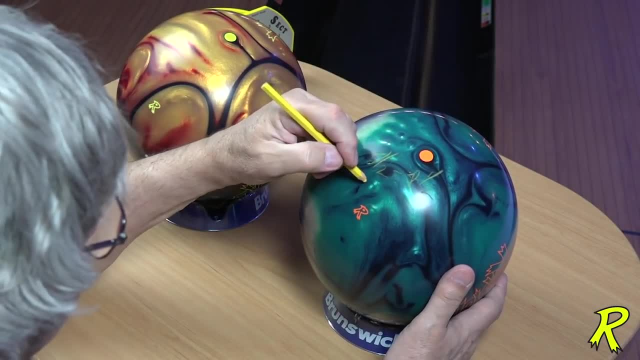 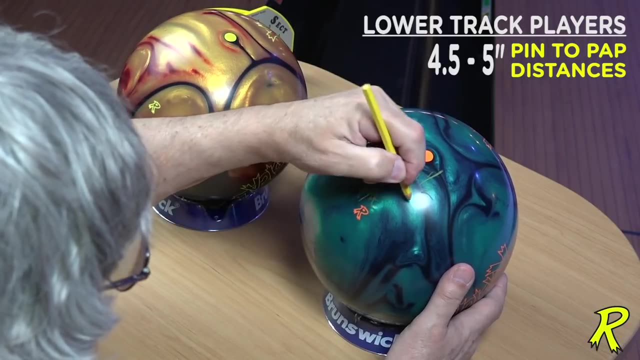 track a little further away from the fingers and the thumb, which means you're going to have more axis tilt. you're going to go between 4 1⁄2 and 5 inches. That's 4 1⁄2.. Okay. There we are. So 3 1⁄2 to 4 1⁄2 if you're a higher track player, 4 1⁄2 to 5 if you're a lower track player. This is because of the amount of axis tilt you have The ball using. 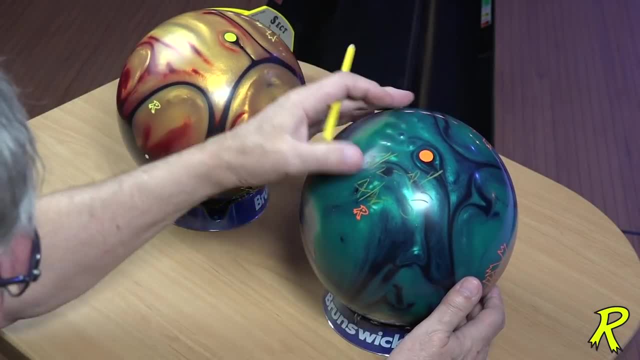 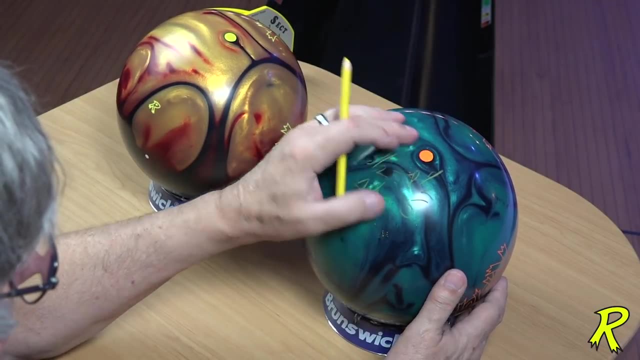 the 4 1⁄2 to 5 inch pin. the pin is going to be rolling over the top of the ball as the ball goes through the mid lane and going to induce forward roll. If you use 3 1⁄2 to 4 inches, the pin is going to be a lot closer to the 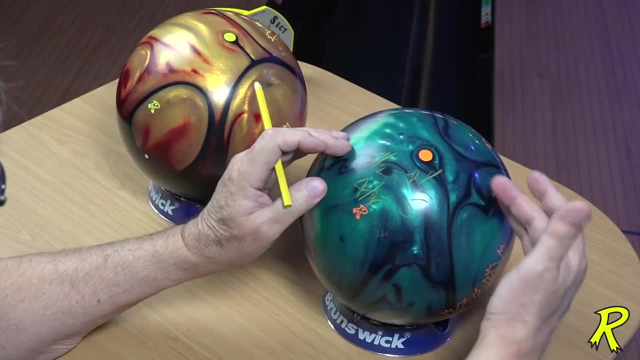 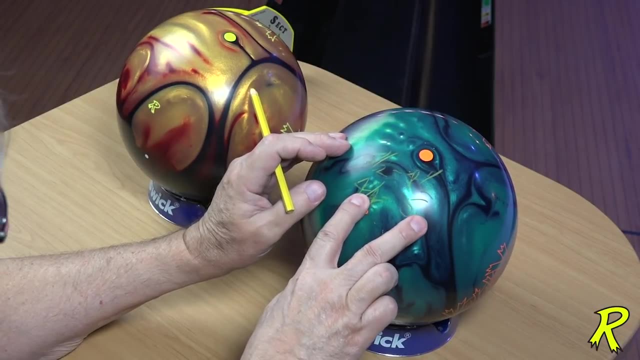 axis point going down the lane and you're going to get more side roll. So side roll 3 1⁄2 to 4 1⁄2, forward roll 4 1⁄4 to 5 inches. So that's where you are on your. 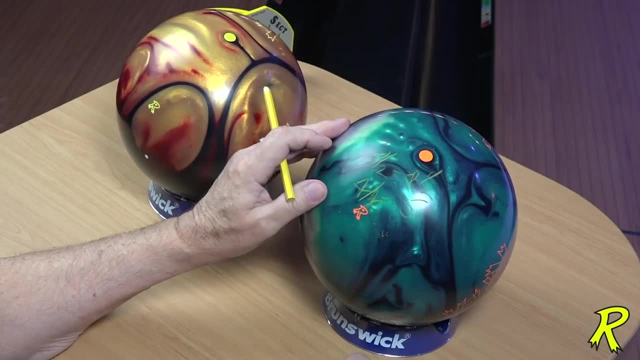 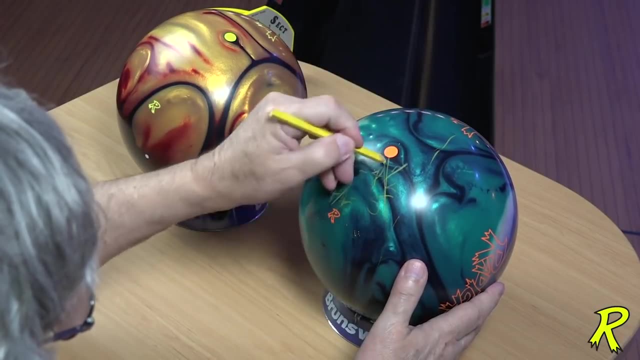 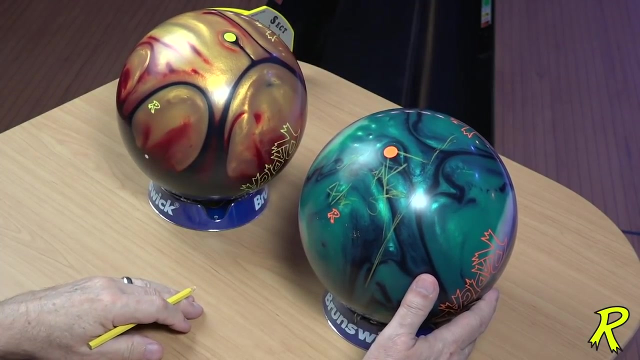 pin to PAP distances. Now let's talk about VAL angles. VAL angles, which is whether the pin is close to the VAL or not. that's this distance right here, which is this angle here, will determine the sharpness of the break point, If you want. 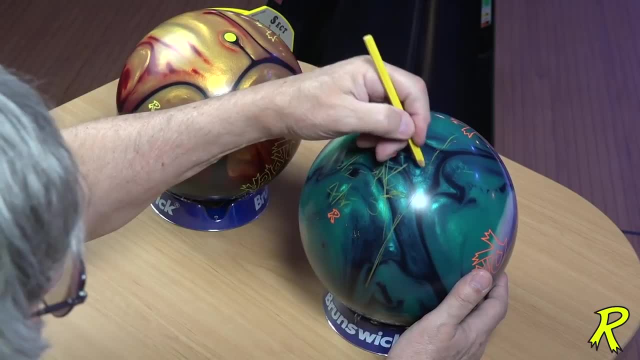 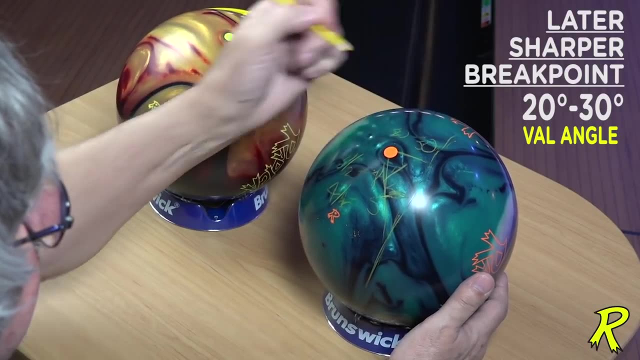 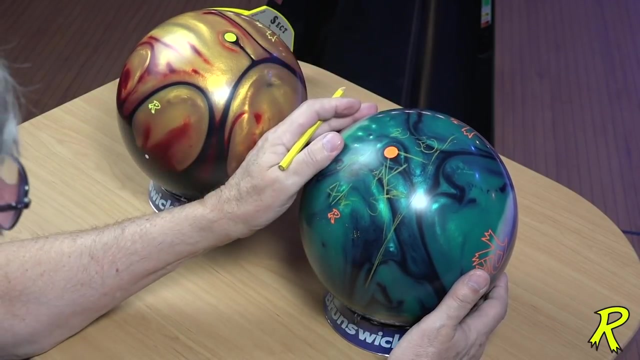 a later, sharper break point. you want the pin closer to your VAL, so you want a smaller VAL angle in the area of 20 to 30 degrees. If you want to see the ball read the mid lane and roll more forward and be more continuous off the spot, you're going to be using VAL. 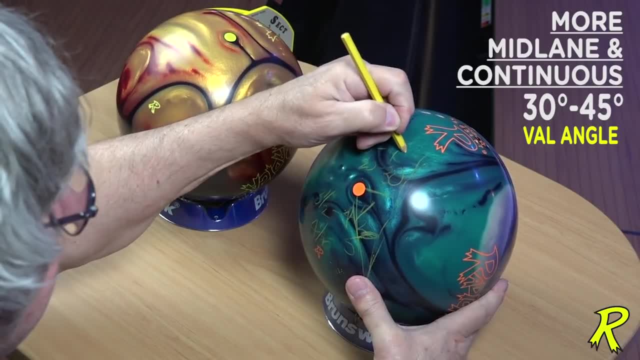 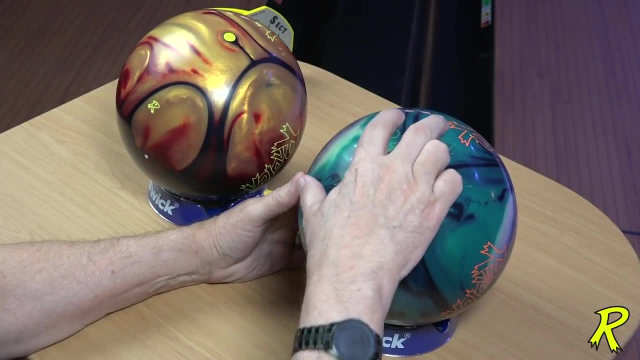 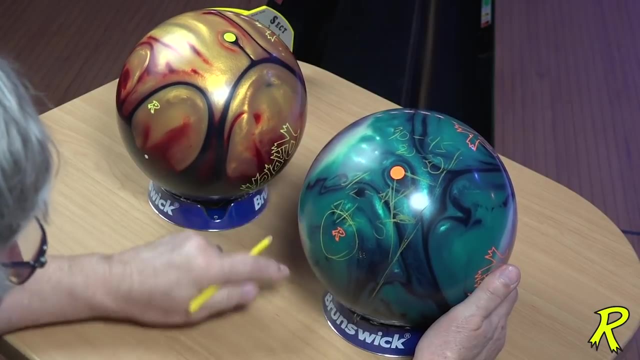 angles of 30 to 45 degrees. So, depending on your style of play, there are two different pin to PAP distances and two different VAL angles. And on symmetrical balls the CG location means nothing because the PSA of the drill ball is going to be in the thumb hole. So 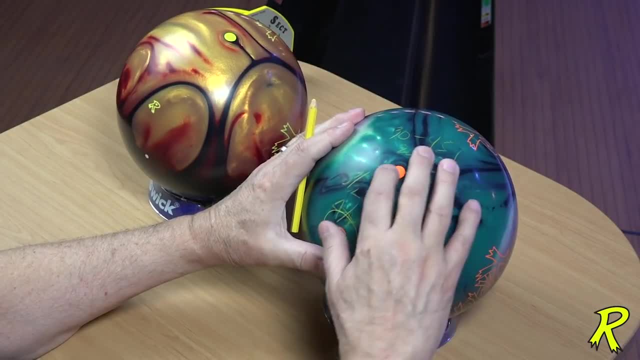 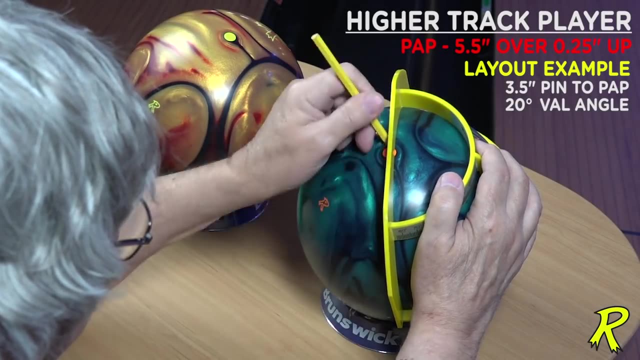 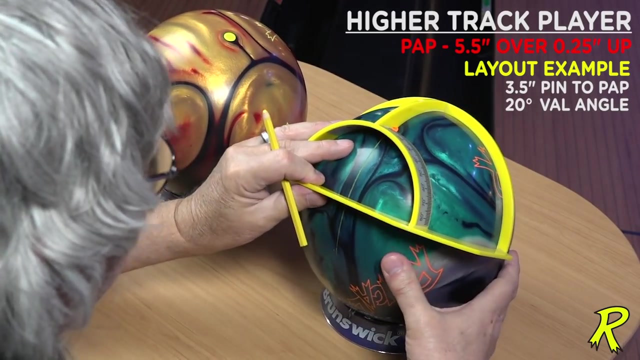 symmetrical balls are kind of symmetrical Subtitles by the Amaraorg community. simple Pin the PAP distance and VAL angle. Here's an example of a layout for a higher track player. I'm going to put the pin three and a half inches from his PAP. I'm also going 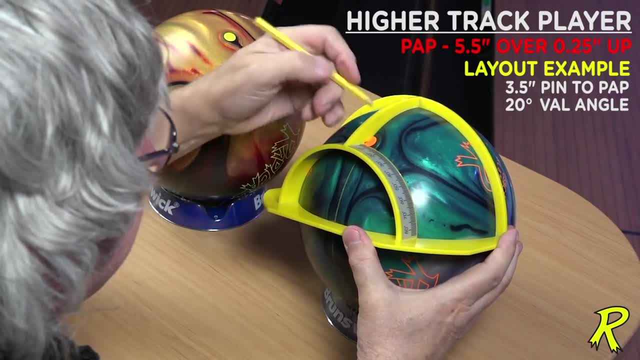 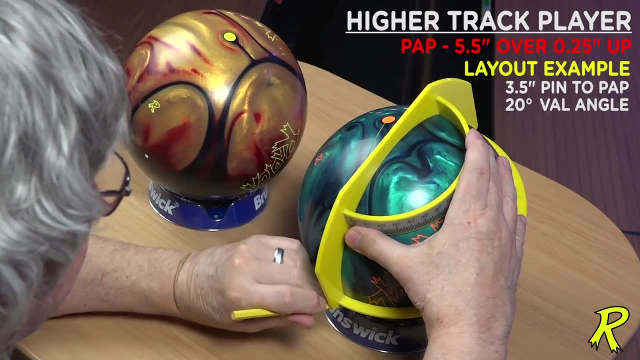 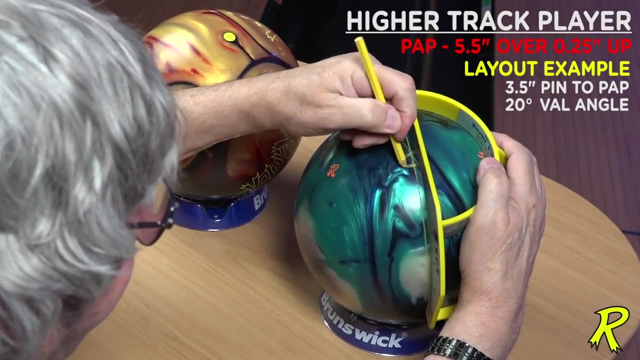 to use a smaller VAL angle: 20 degrees. I'm going to draw the VAL here. I'm using a standard axis point. I'm going to draw the VAL here. I'm going to draw the VAL here I'm going to use a standard axis point, For example as five inches over or five and a half over. 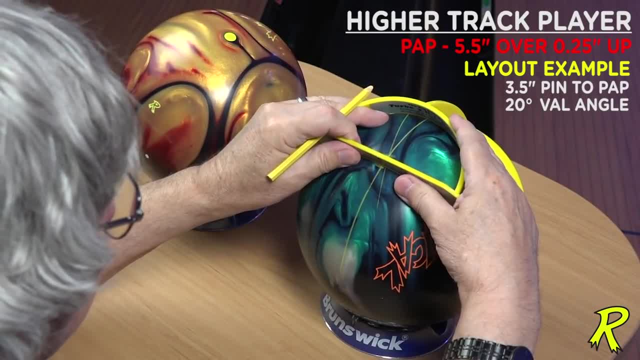 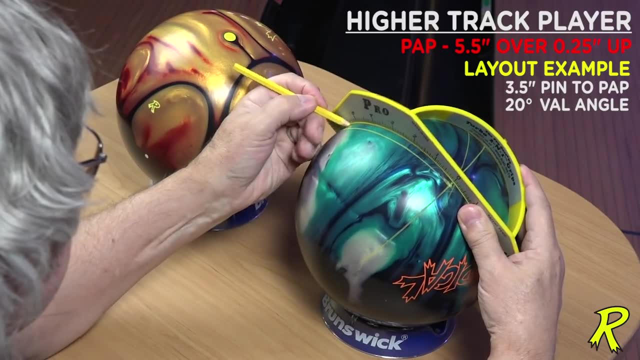 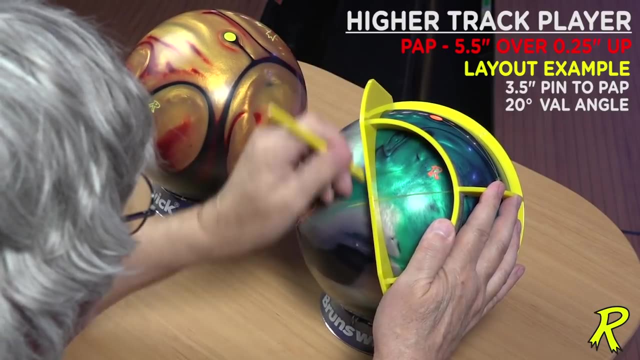 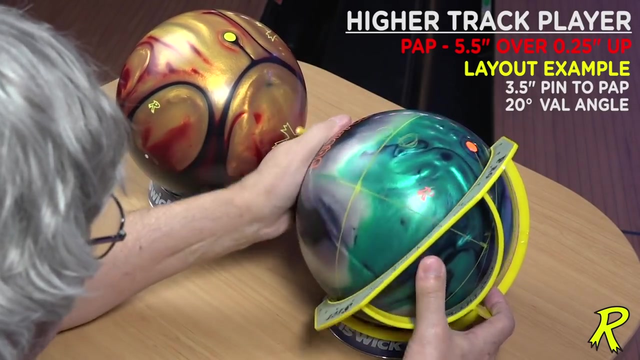 by a quarter up. That would be a typical axis point for a higher track player. Okay, you're looking at a layout similar to this. Put the finger holes here, thumb hole here, third hole there, and there's the layout you're looking for. Easiest way to describe it. 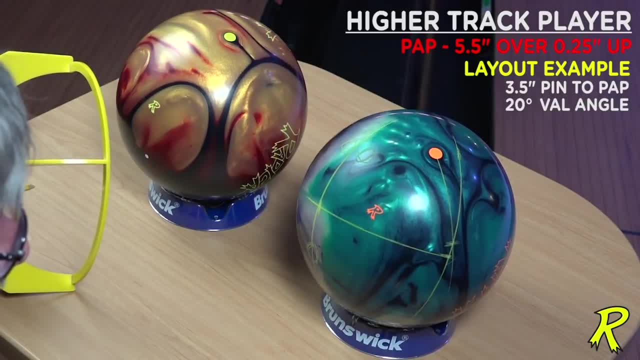 is the pin is up and to the right. That's going to work great for the higher track players, because that's going to give you a break point that's a little sharper and a little later down lane, which is what those people are usually craving. So 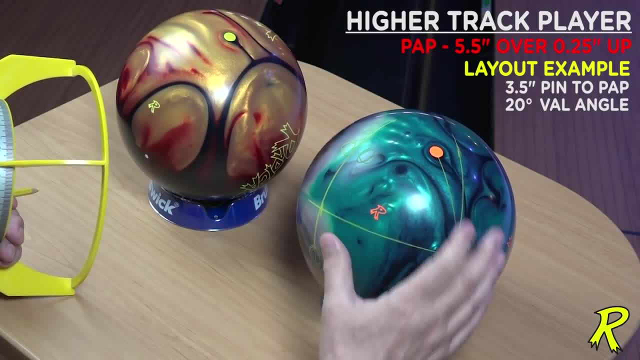 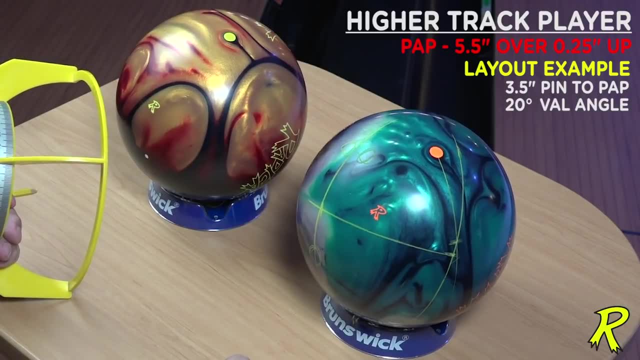 for a later, sharper break point. it's going to look similar to this: This is three and a half pin to PAP, twenty degrees to the VAL. That's going to work great for a higher track player. Okay, now what I'm going to do is give you an. 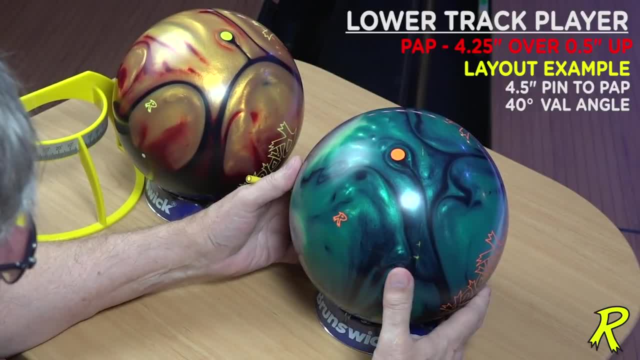 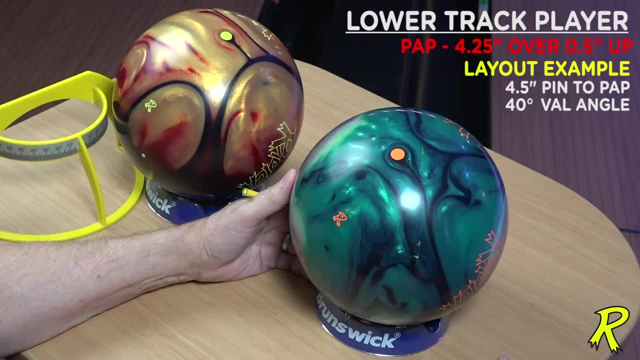 example of a layout on a symmetrical ball for a lower track player. Problem with lower track players are they can't get the ball to read the mid lane well enough, or it's a little uncontrollable on the back end. So in order to do that, 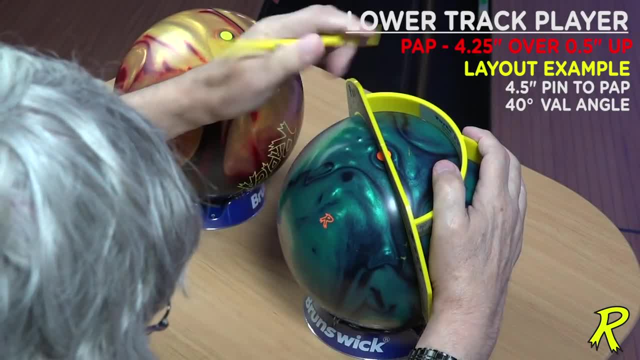 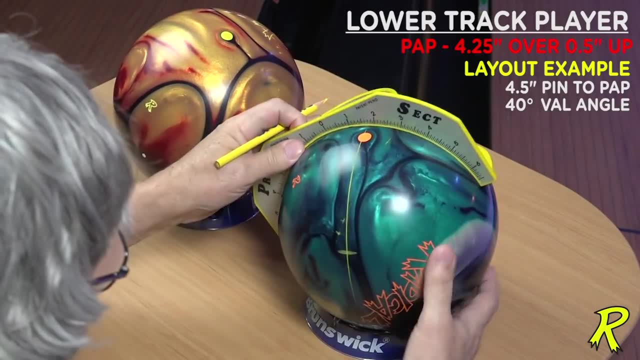 we're going to go to a little bit longer pin to PAP distance, Okay, We're going to get down here to about four and a half inches, Okay, And we're going to use a little bit more VAL angle in order to soften the break point and 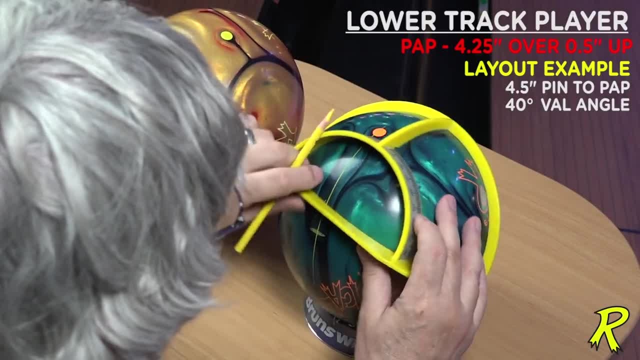 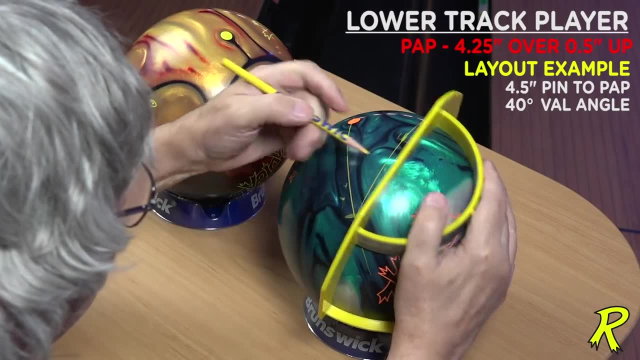 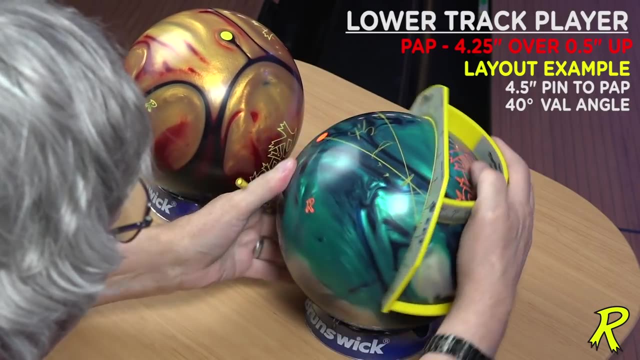 make it a little bit more continuous. So we'll use 40 degrees, Okay, And there's your VAL angle, There's your pin to PAP distance of four and a half inches, Okay, So a typical axis point for a lower track player, and they vary considerably. Moonbee, let's go. 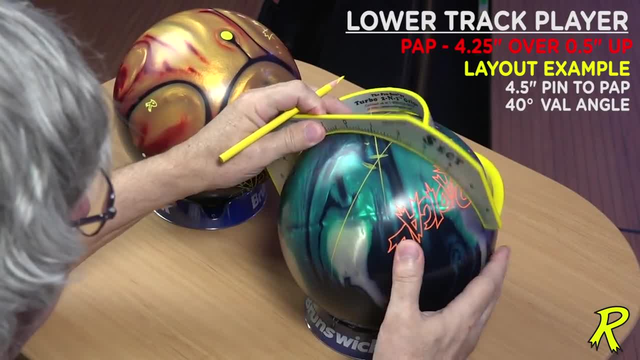 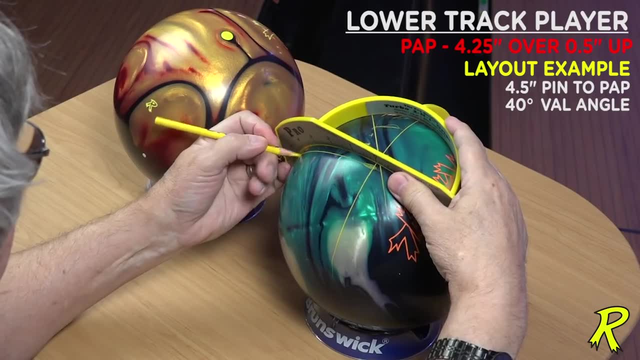 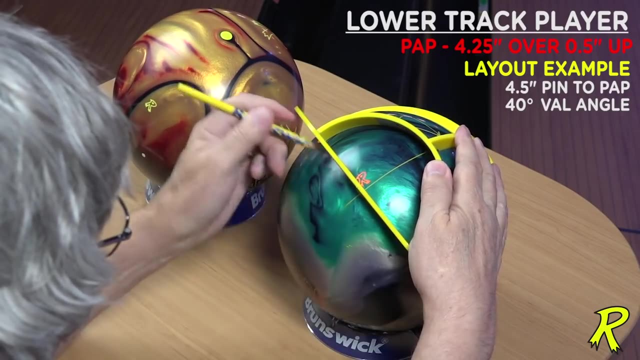 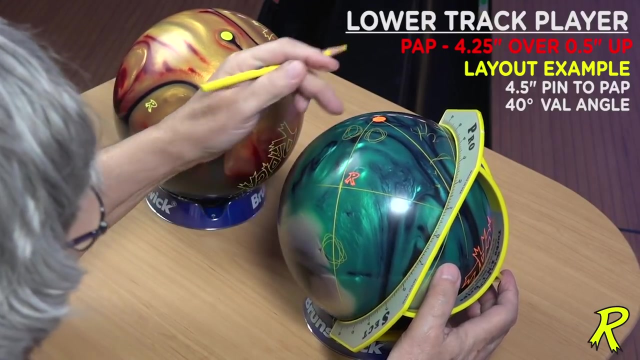 a half down by about four and a quarter over in that area there. Okay, So you're going to get this kind of look. Okay, It's still a pin up ball, but the pin is going to be located more over towards the center line of the grip, above the. 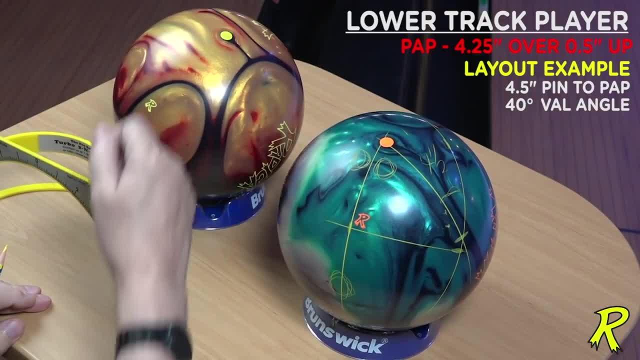 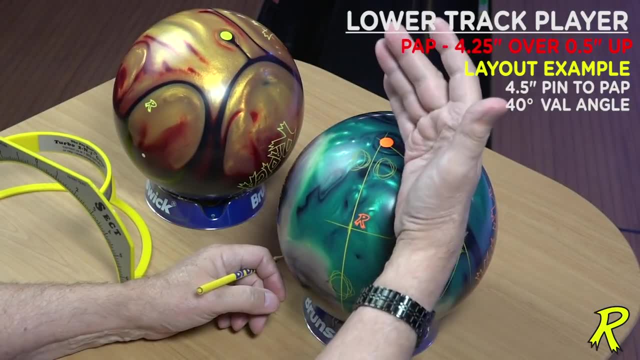 fingers. Now this ball is going to read the mid lane and be more continuous, as opposed to when the pin is up here, and to the right the ball is going to push a little harder and kick a little harder on the back. Pin up and to the right for 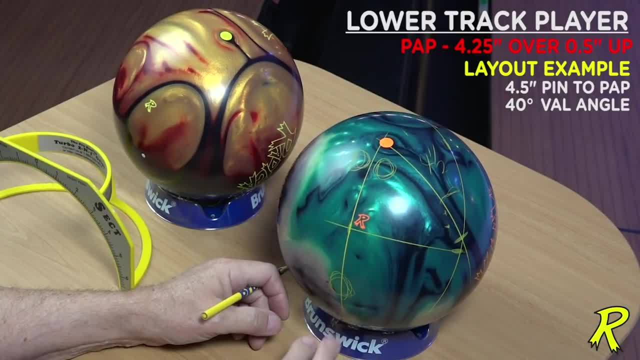 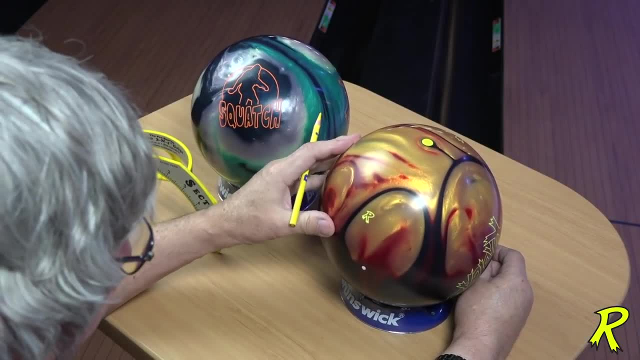 your higher track players. Pin more over the fingers for your lower track players. So that's what you're going to see. Now let's talk about asymmetrical balls. This is a Katana legend. Asymmetrical because it's got a locator pin, The most important factor in layouts for 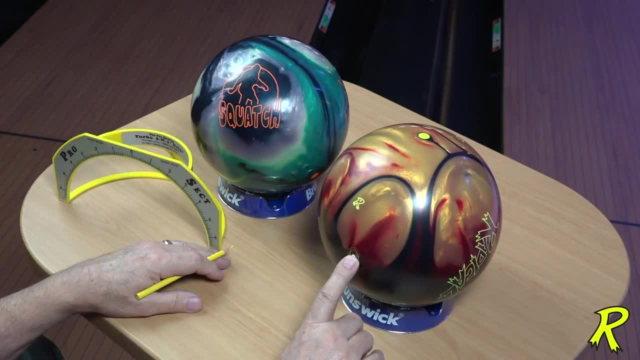 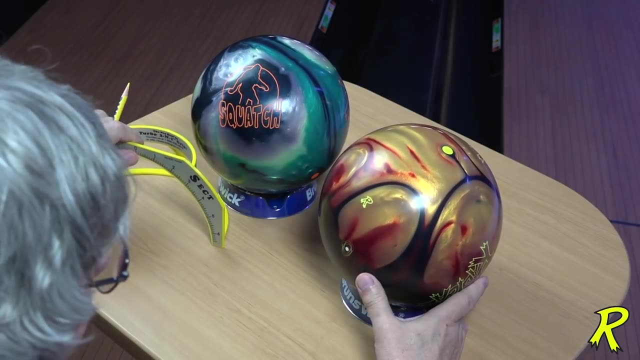 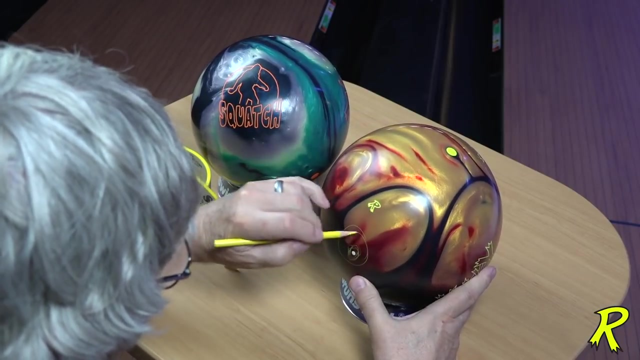 asymmetrical balls is the location of the locator pin in relation to the bowler's axis point. If you want to get the smoothest, heaviest mid lane continuation roll on an asymmetrical ball, you're going to put the locator pin right in the bowler's thumb hole. 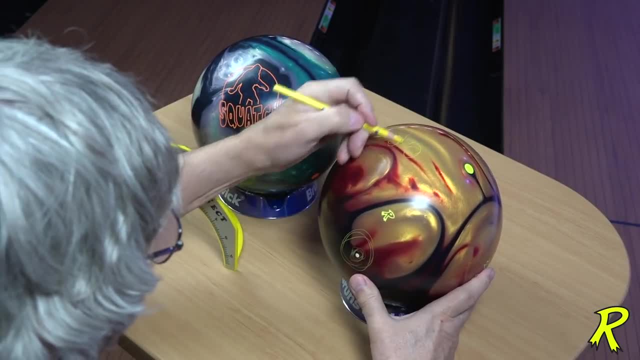 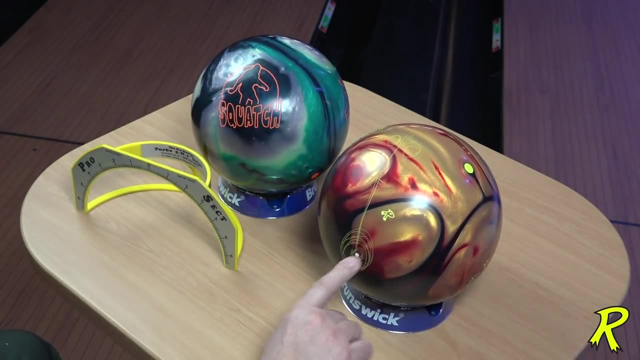 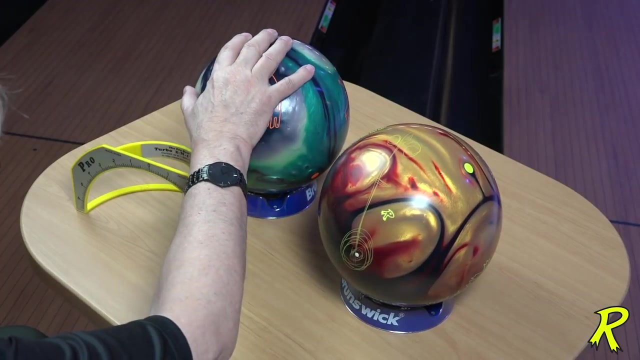 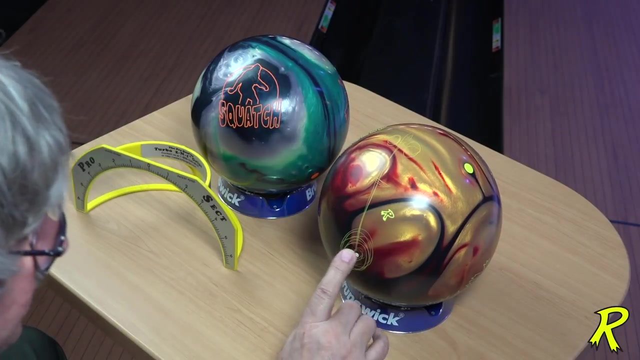 It's going to look something like this, Something like that: Okay, you're going to put the PSA in the thumb hole. This is going to give you a reaction similar to what you used to get with a symmetrical ball with the locator pin in it. It's going to spin where a symmetrical ball spins, but because of 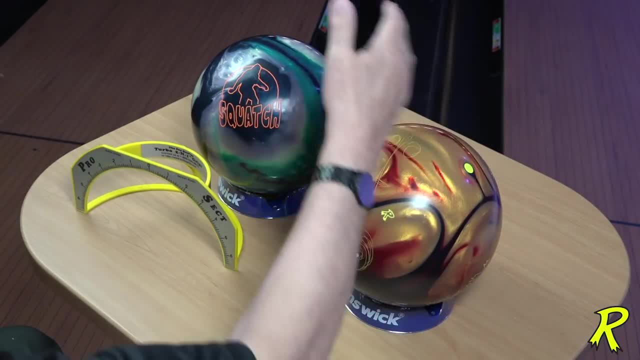 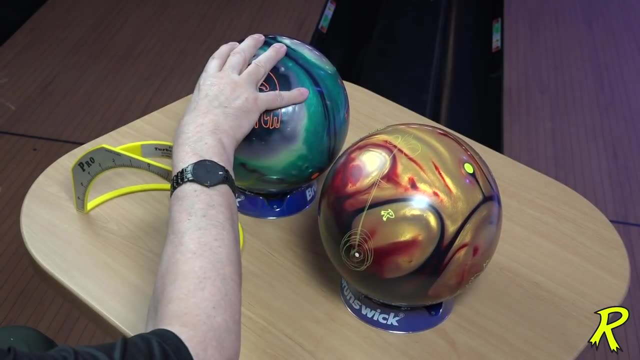 the stronger PSA. this ball is going to read the pattern and continue harder, So this is going to be a stronger ball. The weakest PSA is always more accurate than the counter whenever you use the L rounded ball, the symmetrical ball, because the PSA is in the thumb. Your next PSA location is: 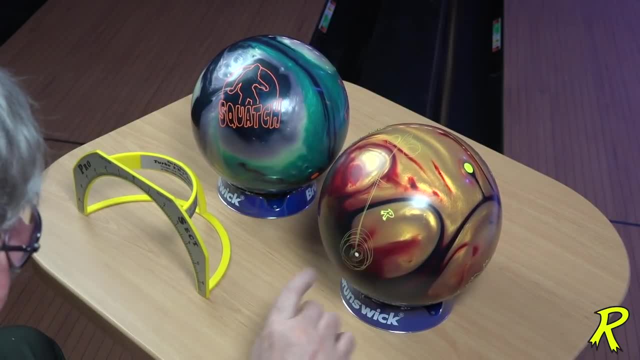 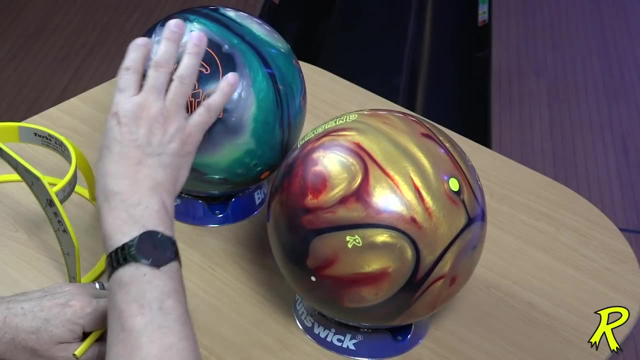 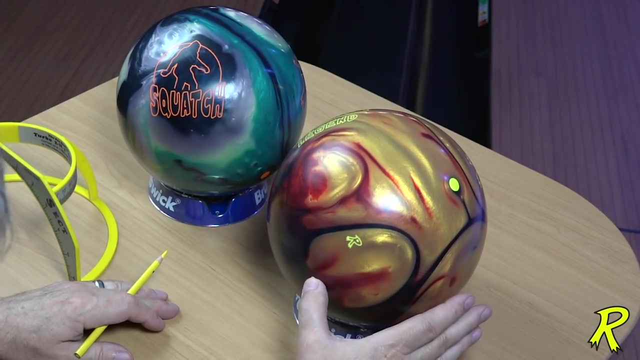 taking a asymmetrical ball and drilling it with the PSA in the thumb. So we've talked about PSA locations. we've talked about the symmetrical ball because PSA is always going to be in the thumb, since we're no longer going to be using balance holes. The next one was a symmetrical ball with the PSA in the 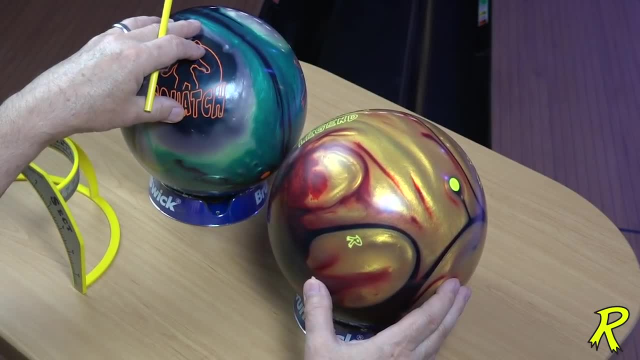 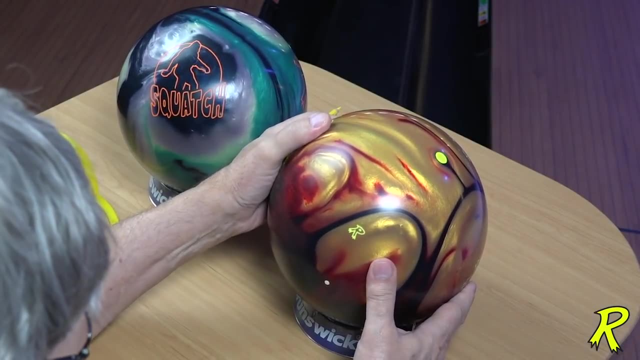 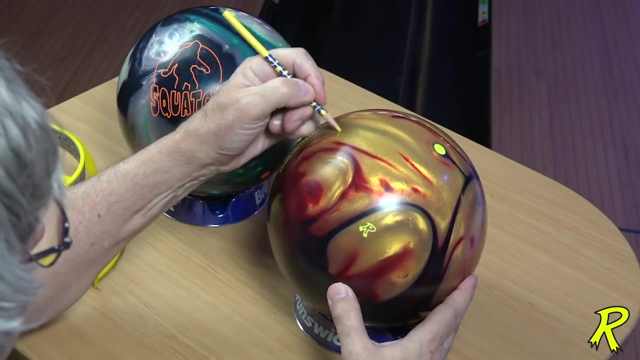 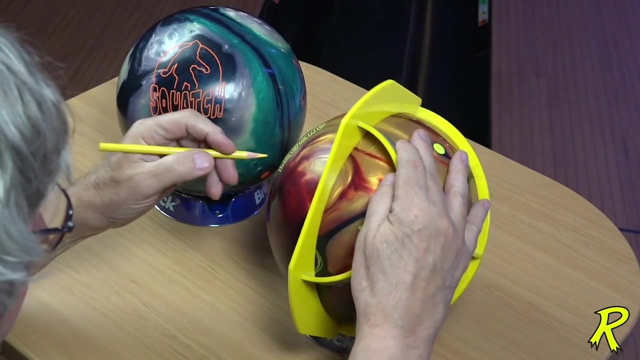 thumb hole That's going to be stronger than the asymmetrical ball, is going to be stronger than the symmetrical ball. Now, if we want to get into a little harder read, we want to move the PSA to the right of the thumb hole for a right-hander. So when you're looking at a layout like this for a 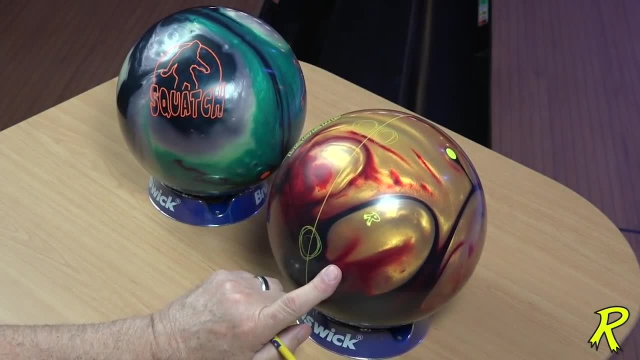 right-handed with the PSA right-of-hand Morgan of the thumb. that's going to get the ball to read the lane a little bit sooner, a little bit firmer. it's going to be harder to throw it through the break point, So symmetrical. 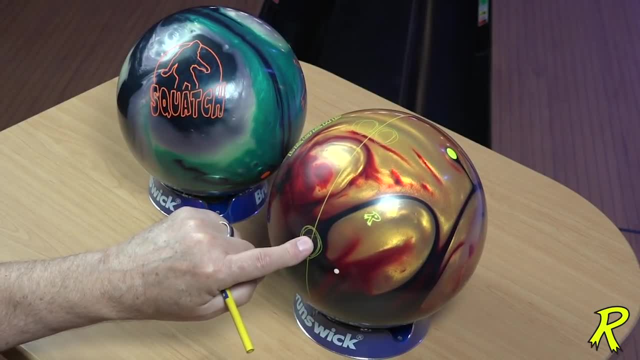 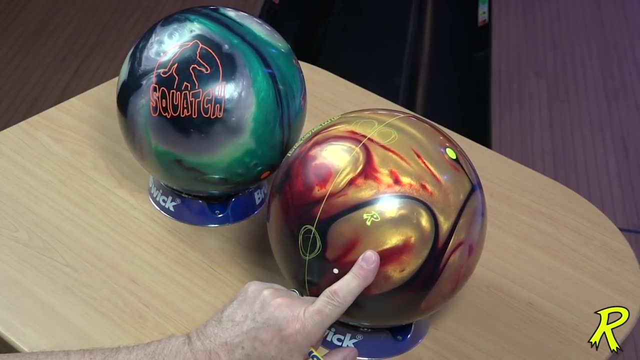 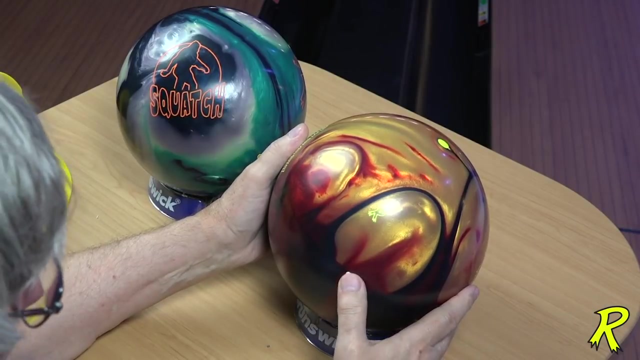 ball- PSA in the thumb, asymmetrical ball- PSA in the thumb and then an asymmetrical ball with the PSA just to the right of the thumb hole for a right-hander. We've talked about three layouts. now let's talk about getting the ball that reads the lane the hardest. 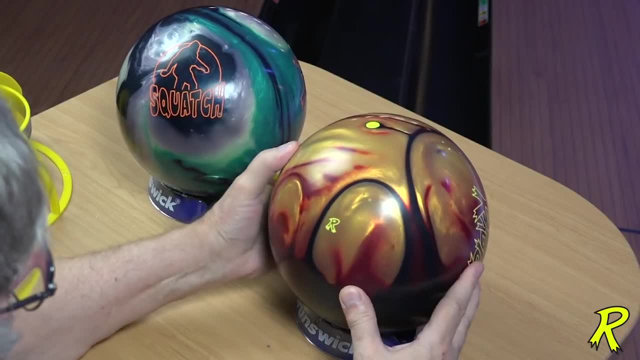 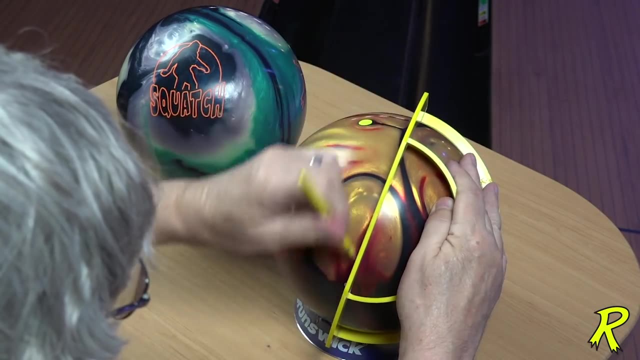 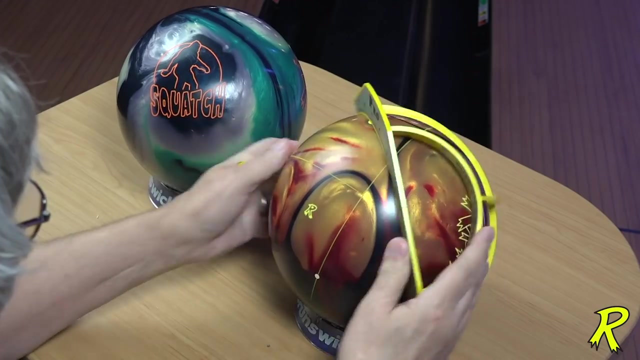 and is hardest to throw through the break point. In order to do that, what we're going to do is we're going to put the PSA on the VAL. That's going to make the ball harder to go through the break point. So the layout's going to look like this: When you want to, 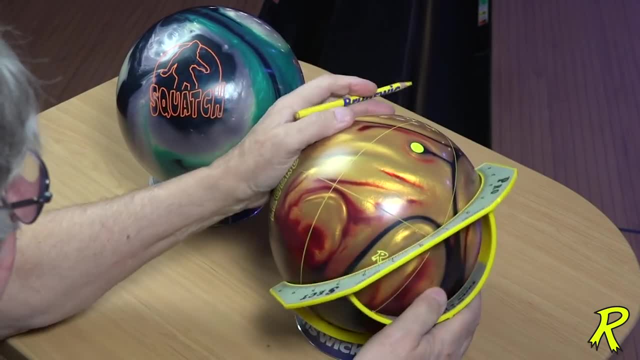 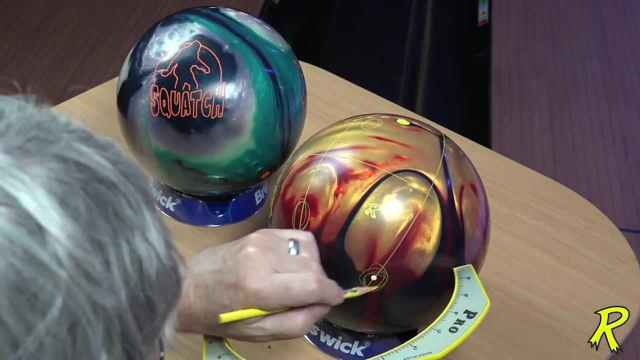 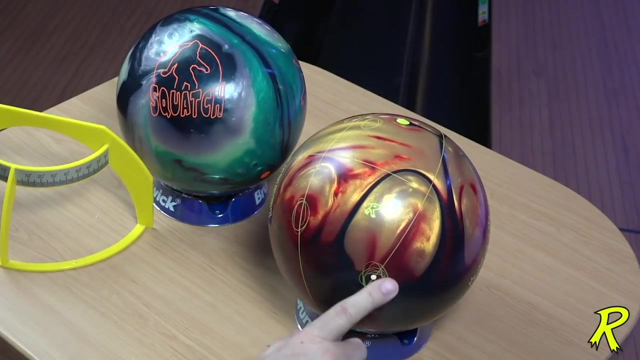 make sure you can't throw the ball through the break point and you want to get the firmest read to the oil pattern? Okay, PSA over there on the VAL. So asymmetrical balls are more versatile than symmetrical balls because you can move the PSA around. You're going to get the softest reaction with. 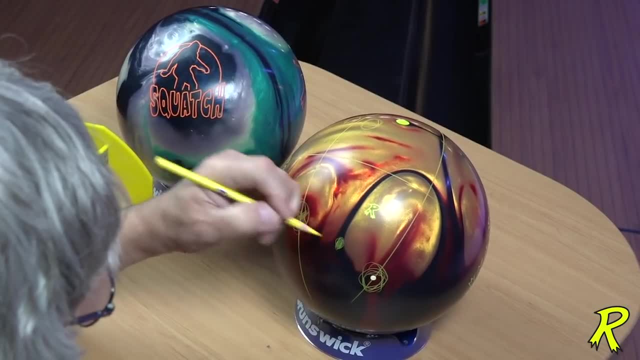 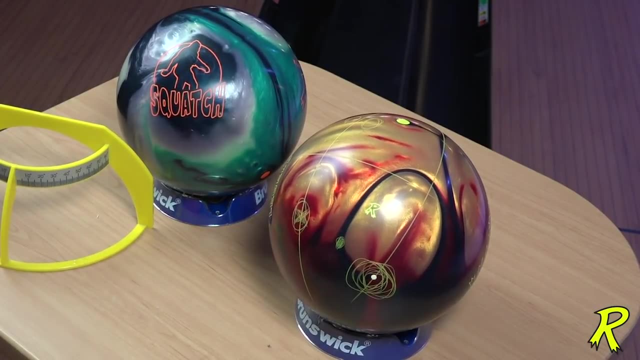 the PSA in the thumb, you're going to get the medium reaction with the PSA between the thumb hole and the VAL and you're going to get the ball that reads the pattern the best with the PSA on the VAL. So PSAs on the VAL. 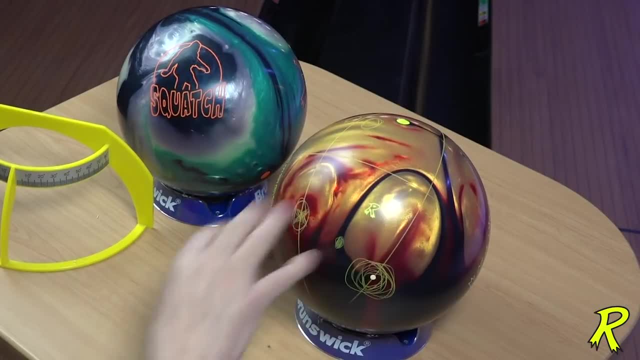